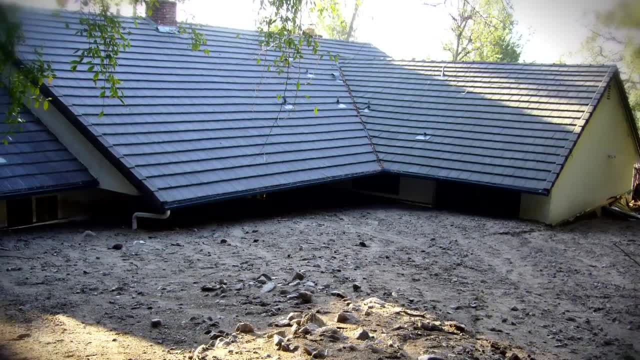 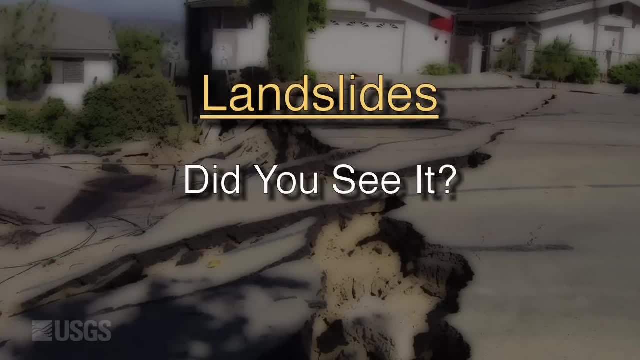 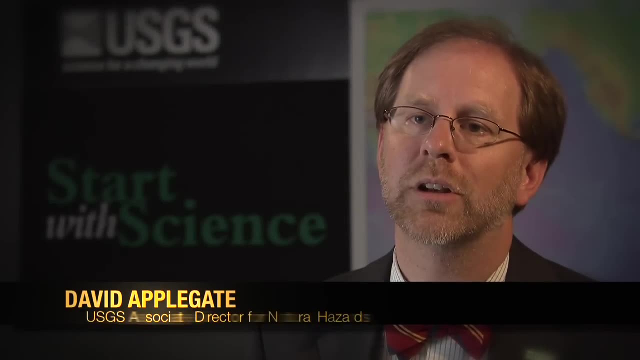 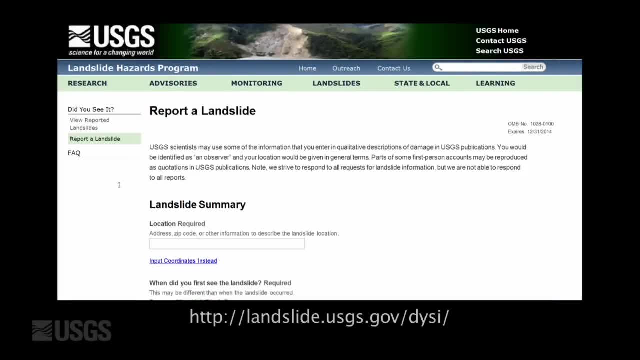 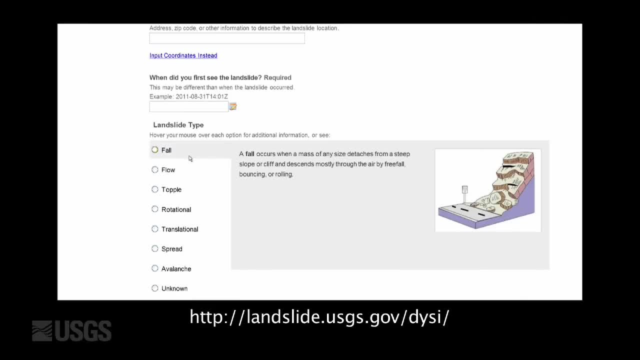 in which members of the public can come to our website and give descriptions of the landslide, the characteristics of it. Hopefully we'll even be able to post photographs of it And we'll start to build a database that will be very useful to us scientifically. 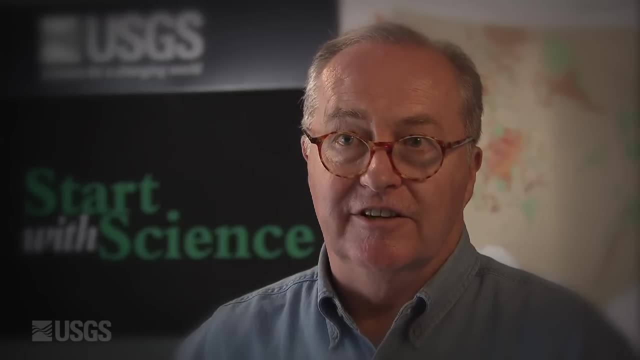 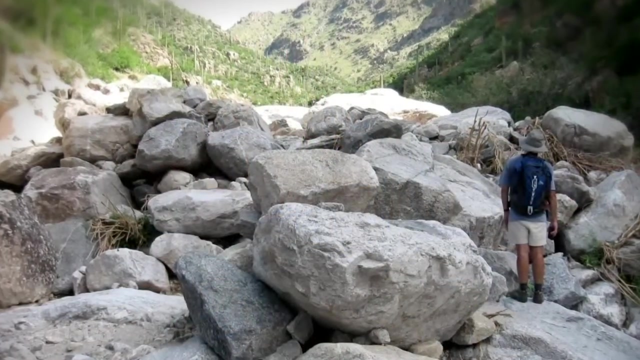 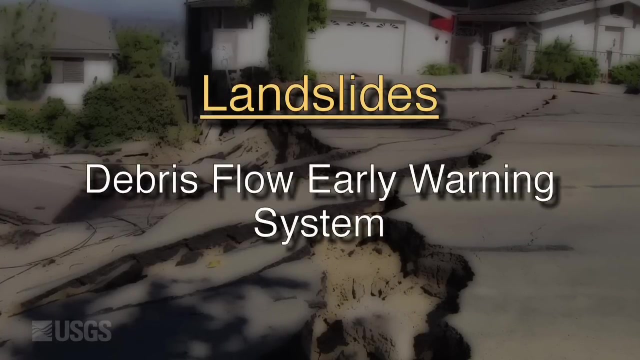 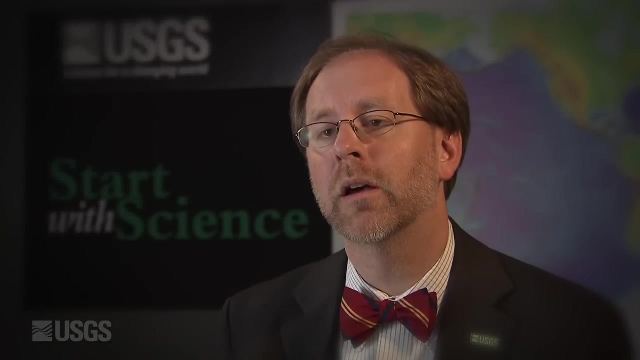 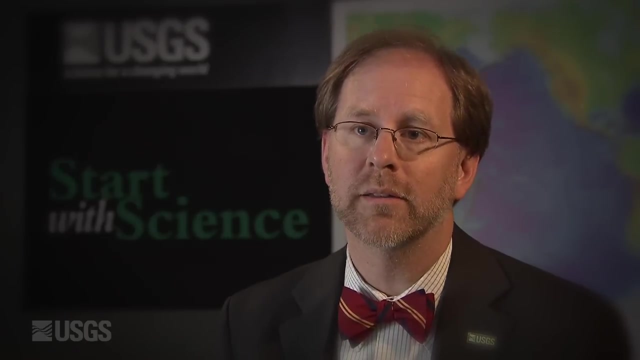 Hundreds of thousands of landslides occur in the United States every year, Of every imaginable, Every imaginable scale. We would like to ultimately someday have an inventory of all those landslides. In the area of landslides, we've been working with partners in the National Oceanic and Atmospheric Administration's National Weather Service on a debris flow early warning system. 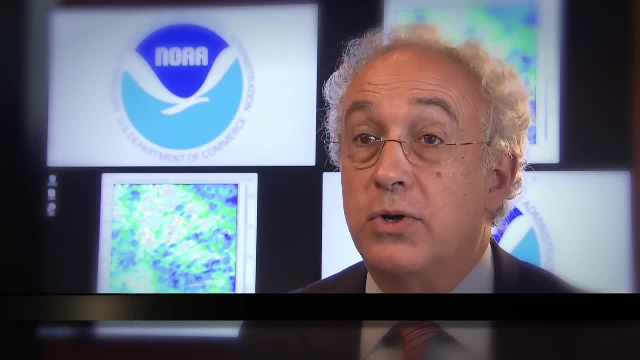 In the area of landslides, we've been working with partners in the National Oceanic and Atmospheric Administration's National Weather Service on a debris flow early warning system. The collaboration between NOAA and the URGS has resulted in a warning system that is helping the people. 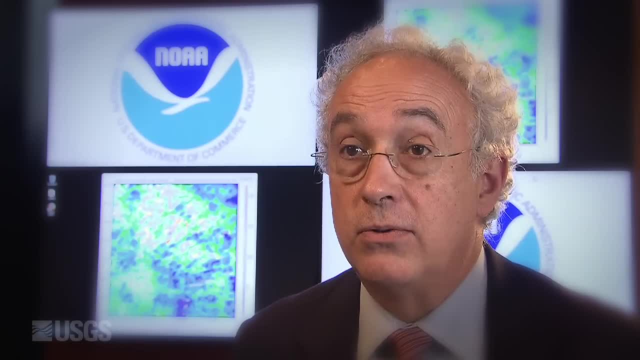 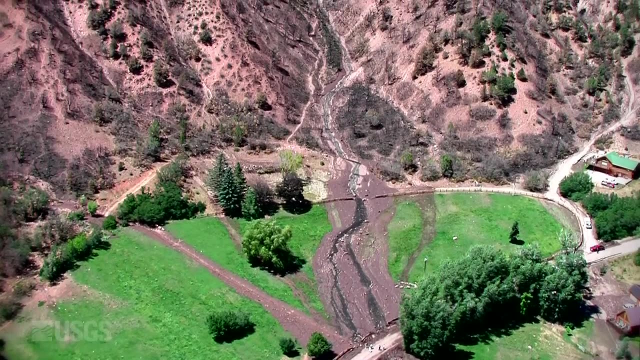 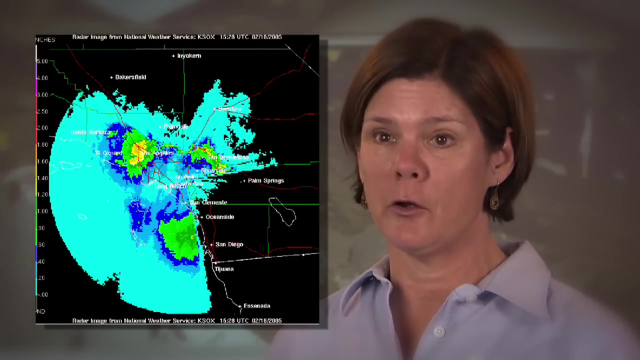 in the communities that are susceptible to debris flows is, within Southern California, to be safer and to be more resilient. Within this warning system, the weather service takes the role of issuing the forecasts and measuring what sort of rainfall is occurring, And then they have the system for disseminating watches and warnings. 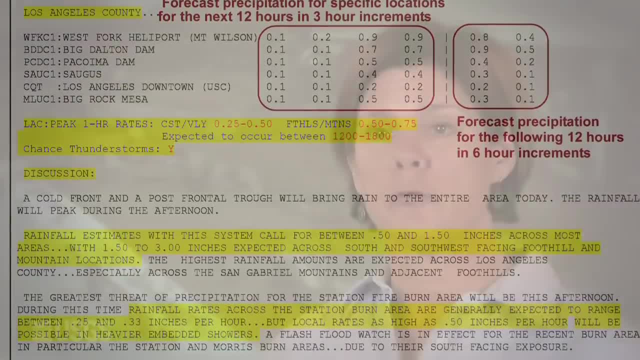 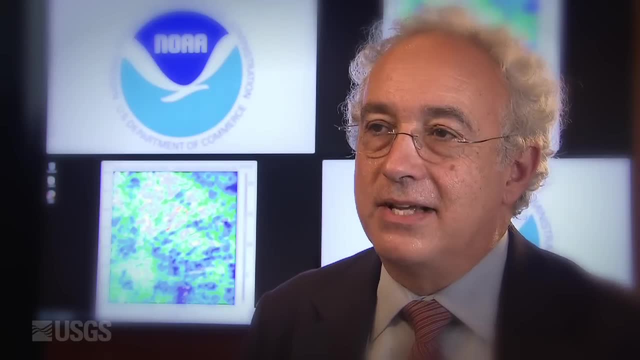 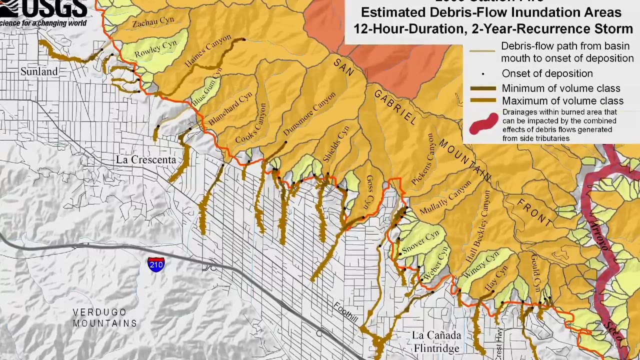 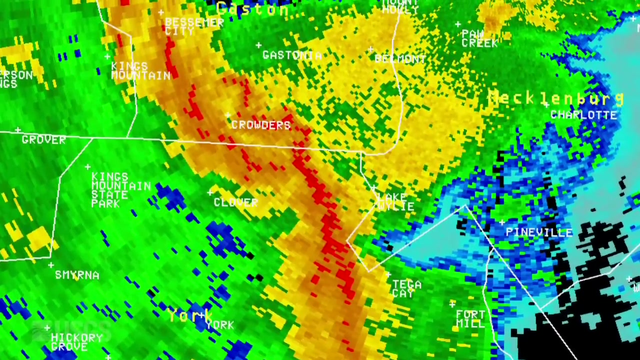 The USGS brings to the table our knowledge about what sort of rainfall conditions will lead to the landslides and what areas would be the most susceptible. The debris flow warning system involves for the National Weather Service to use models developed by the geological survey and in combination with our own observations using high-resolution radar and weather forecasts.